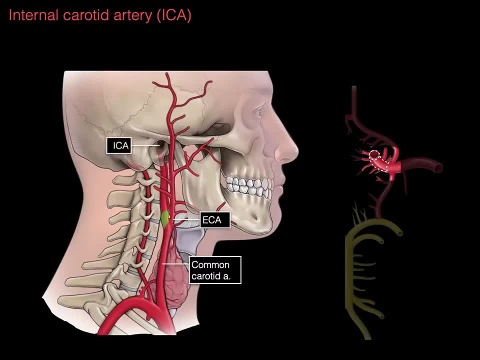 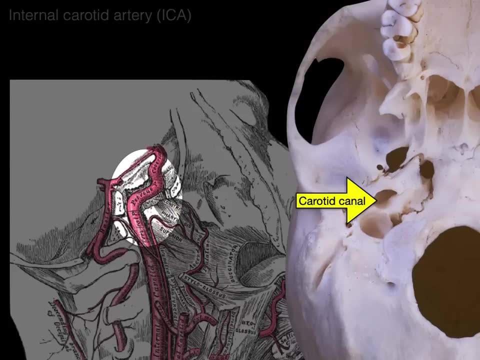 the internal carotid artery. the internal carotid artery ascends up and then goes through the base of the skull, And so there's that base of the skull where the carotid canal is, And so if we zoom in, there's our internal carotid artery and the carotid canal, and both on the bottom and in. 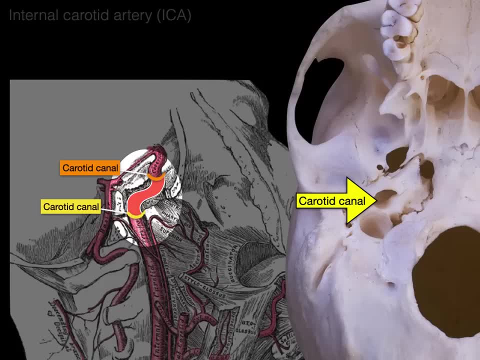 the cranial base and there's the carotid canal in which the internal carotid artery traverses. So we notice that there's a part of the internal carotid artery in the neck, the cervical region, in the carotid canal, the petrous region in the cavernous sinus. 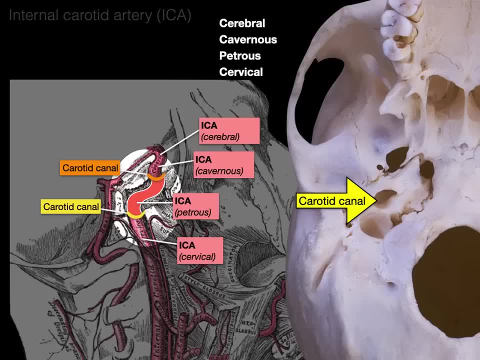 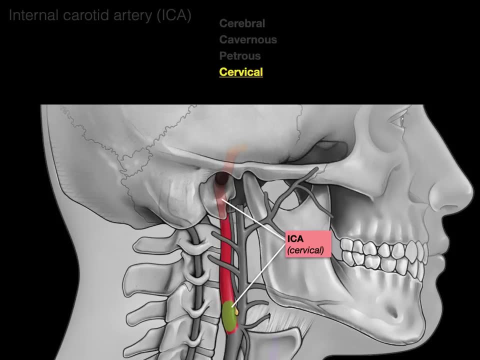 and then that's supplying the brain. So there's basically these four parts to the internal carotid artery. Let's do it again. The cervical part of the internal carotid artery is in the neck. what's shown there? that's highlighted the cervical region. Then there's the petrous part. 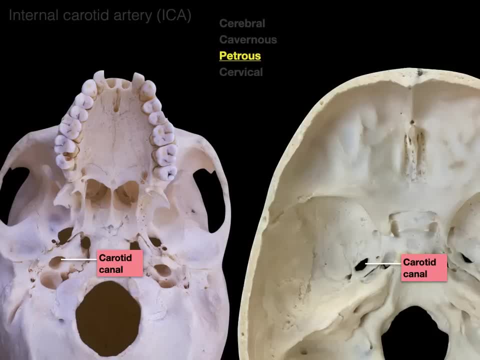 which is going from the carotid canal on the base of the skull to the carotid canal in the middle cranial fossa. Between the two is the internal carotid artery, the petrous part. Then the cavernous part is the part that's in. 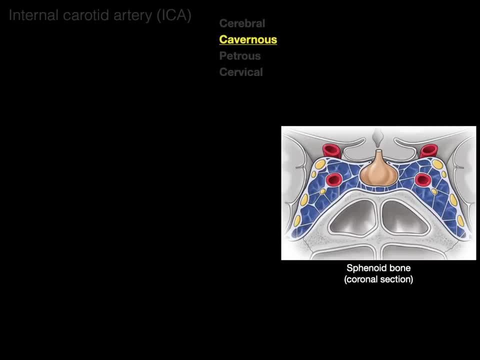 the cavernous sinus. So there's a sphenoid bone in a coronal section. In blue is the cavernous sinus, one of the dural venous sinuses flanking either side of the pituitary, And there's the 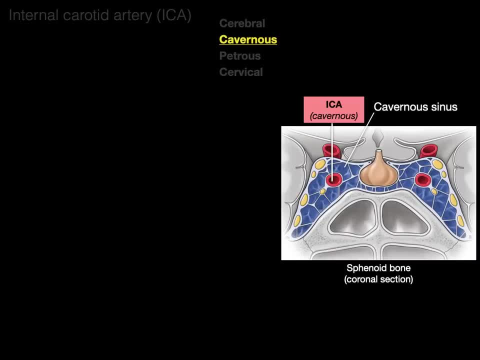 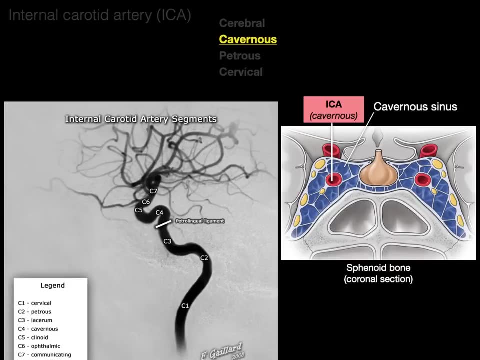 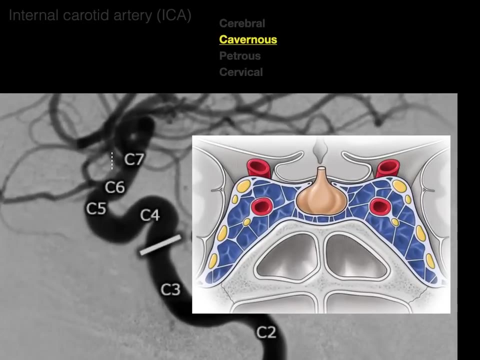 internal carotid artery, the cavernous portion, the only prime in anywhere in the body where you see an artery inside of a vein. It's very cool. So let's take a look at this angiogram where you inject a dye into the internal carotid artery and then take an x-ray of it, where, if we zoom in, 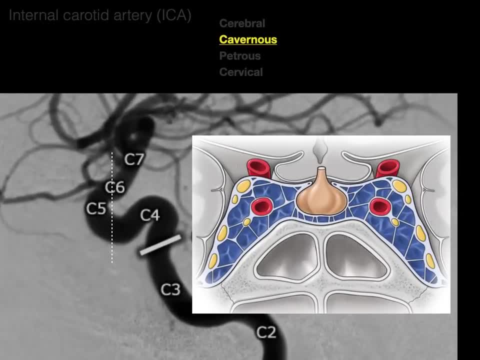 and take a coronal section through this lateral view of the internal carotid artery. there is the internal carotid artery in the cavernous sinus, But watch, it goes and it curves around. And then, if we take another cross-section, there is the cerebral part. 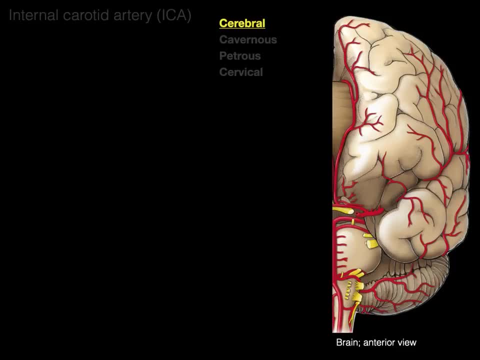 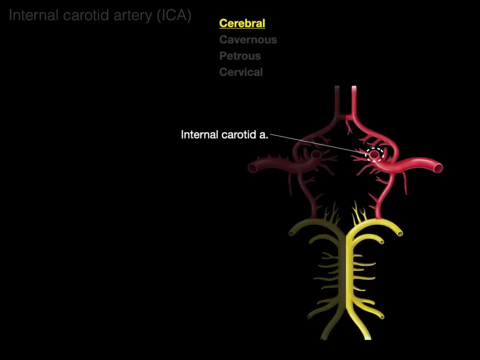 of the internal carotid artery And basically the cerebral part is that part right there where all the other branches that we're going to talk about come off. There is the internal carotid artery, the cerebral part, And one of the major. 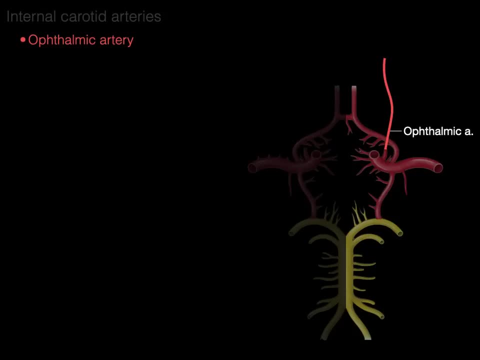 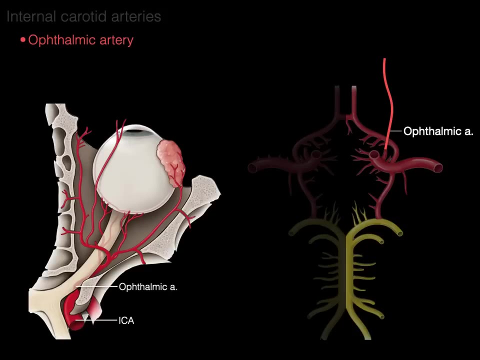 one of the branches that comes off is called the ophthalmic artery And, as its name implies, goes to the eye. So there is a superior view of the orbit, our internal carotid artery. There's the ophthalmic artery, going in through the optic canal and gives rise to all these. 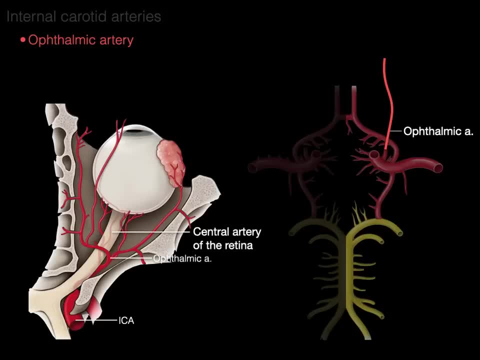 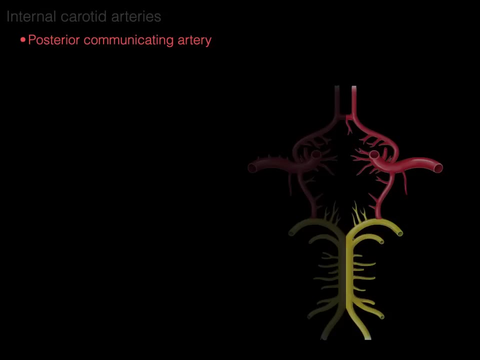 arteries that go into the orbit And clinically a really important one is the central artery of the retina. that supplies arterial supply to the retina And if it's occluded because of diabetes or a clot then blindness or vision problems occur. Another artery that comes off the internal carotid is called the posterior communicating artery. 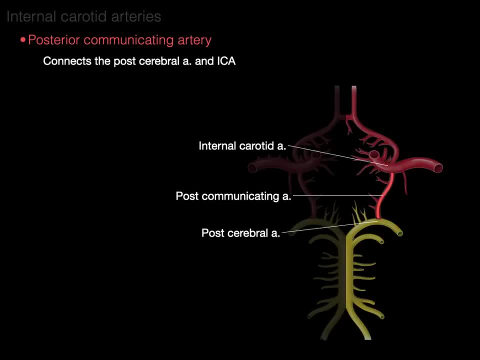 that connects the posterior cerebral artery and the internal carotid arteries. It also connects our anterior and posterior circulations. on one side There's our anterior circulation of the brain and there's the posterior circulation of the brain, And the posterior communicating arteries connect the two together. They're paired one on either side. 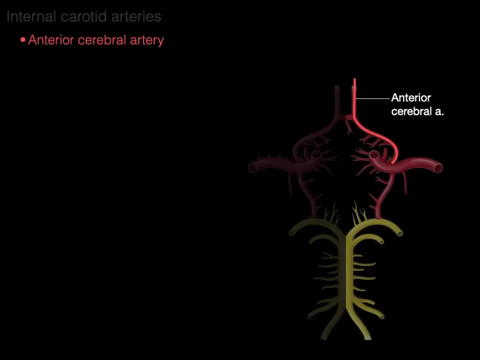 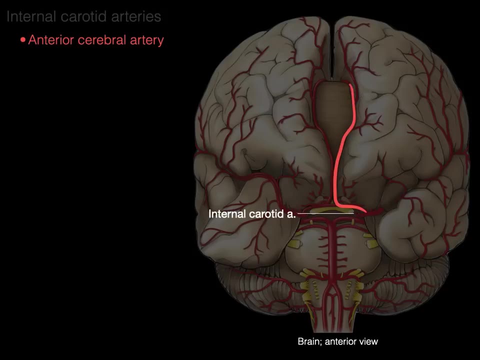 Then there's the anterior cerebral artery right there that supplies the front of the cerebrum. So here's the front of the cerebrum and there's our internal carotid and there is one anterior cerebral artery coursing over top of the corpus callosum, within the 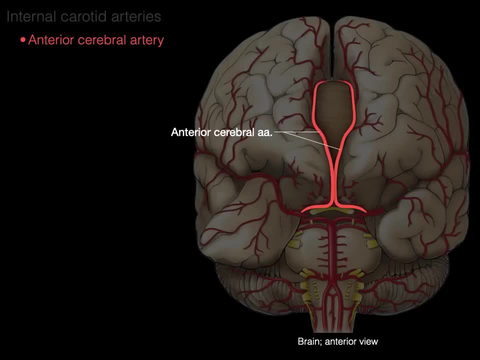 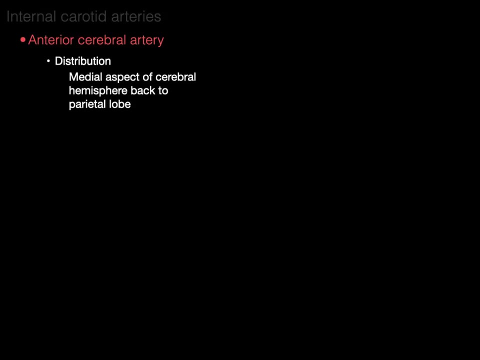 longitudinal cerebral fissure And it's paired. the anterior cerebral arteries are paired. okay, The distribution of the anterior cerebral artery is the medial aspect of the cerebral hemisphere, all the way back to the parietal lobe. Let's see what that looks like. Okay, I'm going to make the 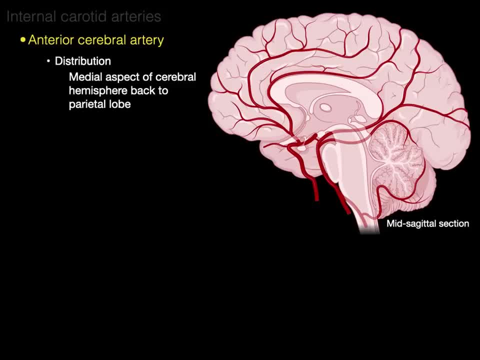 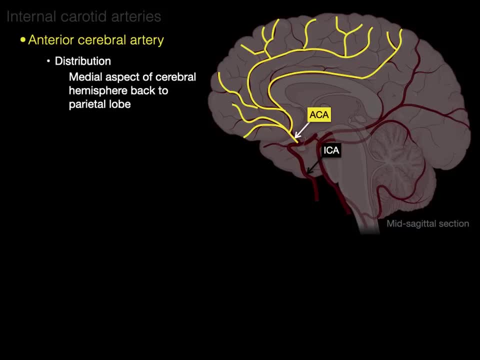 anterior cerebral artery look yellow, because that's the picture I'm going to show is in yellow. So here's a mid-sagittal section of the brain, There's our internal carotid and there's our anterior cerebral artery, And there is the anterior cerebral artery coursing over the 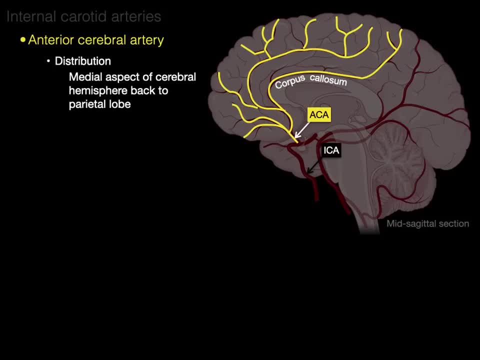 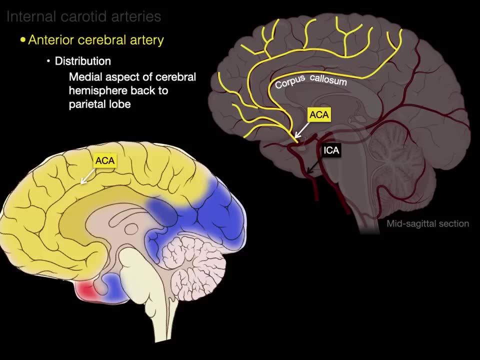 corpus callosum and you can see its distribution okay, Right in the midline of the brain. And so here's a mid-sagittal section of the brain, and everything you see in yellow is supplied by the anterior cerebral artery, the medial aspect of the cerebral hemisphere, all the way back to 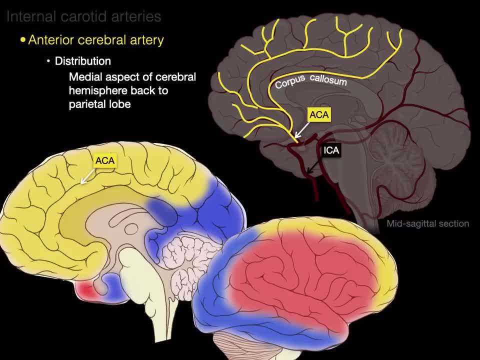 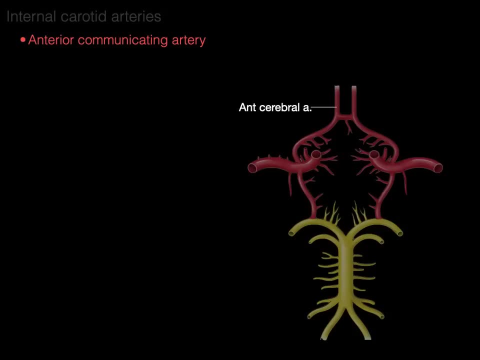 the parietal lobe And even in this lateral view of the right side of the brain, there you can see the anterior cerebral artery is supplying the medial aspect of the cerebral hemispheres back to the parietal lobe. All right now, the anterior communicating artery is between our two. 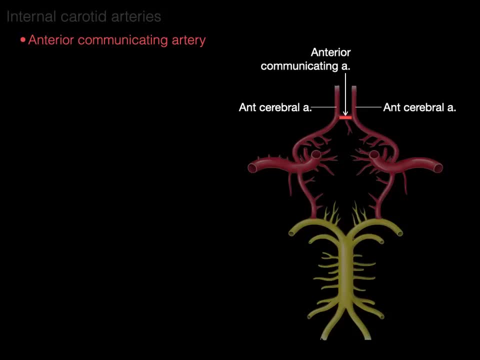 anterior cerebral arteries. right there, our anterior communicating artery. Let's do that again. from this anterior view. There are showing our anterior cerebral arteries and shing whoops and shing. right there is our anterior communicating artery connecting the two together. 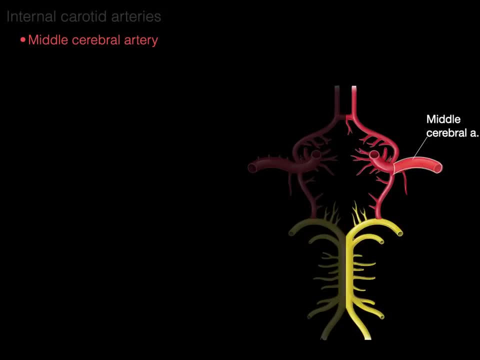 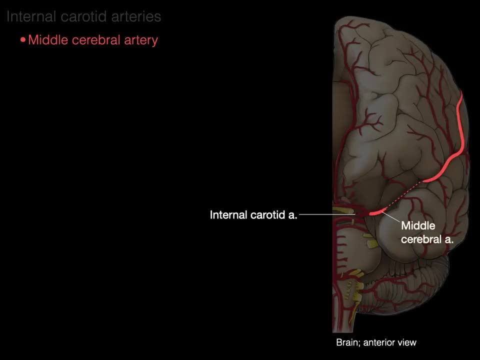 Now our middle cerebral artery is right there And middle cerebral because it's the middle of the cerebrum. So here's the brain in anterior view, There's our internal carotid artery and there is our middle cerebral artery right within that lateral sulcus, And so the distribution is. 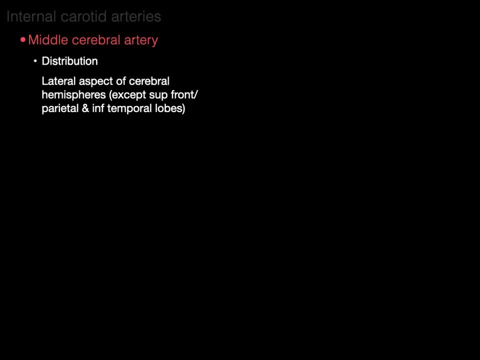 through the lateral aspect of the cerebral hemispheres, except for the superior portion of the frontal and parietal lobe, And so the lateral aspect of the cerebral hemispheres is for the anterior cerebral artery and for the posterior cerebral artery And for the inferior. 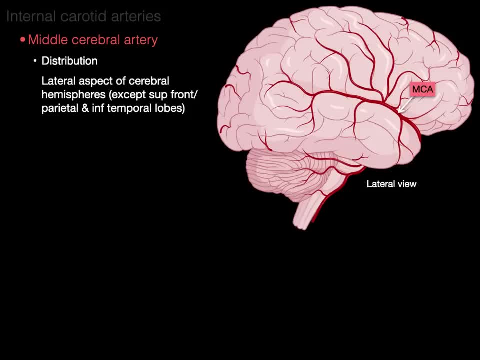 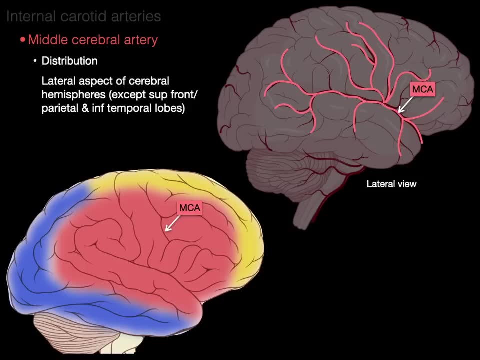 part of the temporal lobe. Let's see what that means. Okay, so here's the lateral view of the brain. There's our middle cerebral artery and there's its distribution, And so, if we look at this picture again, there's the. everything in pink is showing the distribution supplied by the 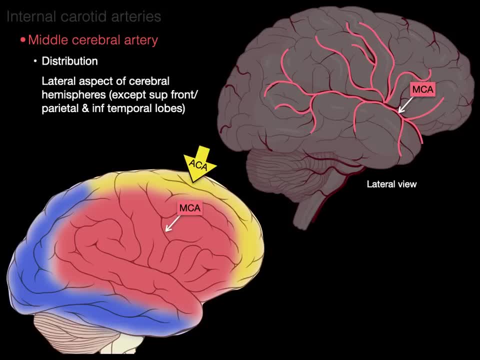 middle cerebral artery, all except the superior portion of the frontal and parietal lobes and in the inferior portion of the temporal lobes And you can see, the anterior cerebral and posterior cerebral arteries supply those two areas Now let's focus on. there's our internal carotid artery. 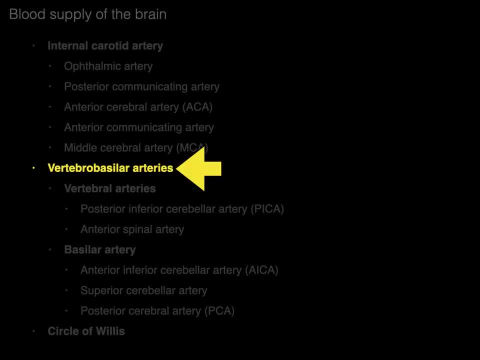 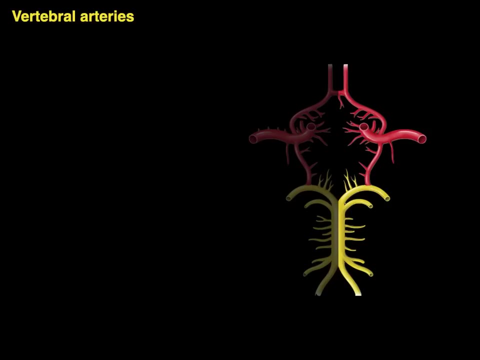 Now let's go to the vertebral basilar arteries, and they're consisting of the vertebral and the basilar arteries. So now let's take a look at the vertebral arteries and its branches. So the vertebral artery is located there. 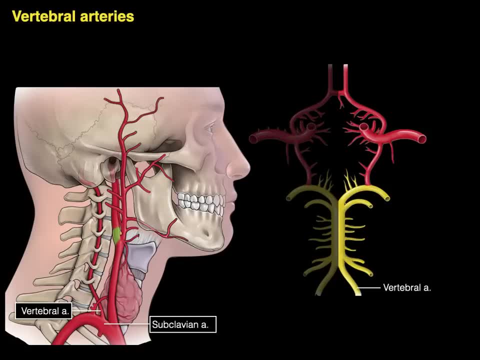 It's paired, one on either side, and it arises from the subclavian artery and it ascends up the neck through the transverse foramina of the cervical vertebrae, through the foramen magnum and into the skull. 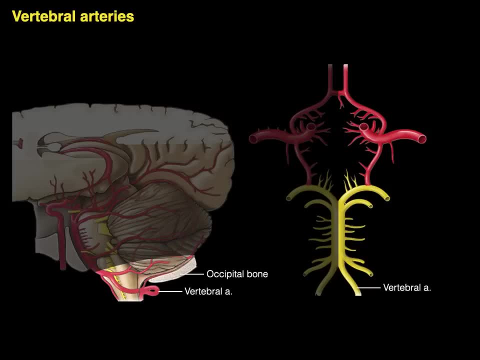 And so there is the vertebral artery, There's the base of the skull, the occipital bone. There, in dashed line I've added the foramen magnum, and the vertebral artery comes up, traverses the foramen magnum, fuses with the other vertebral artery and they become the 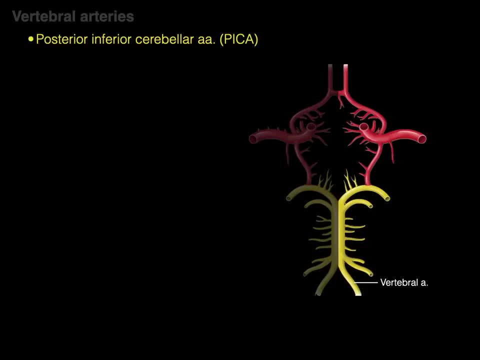 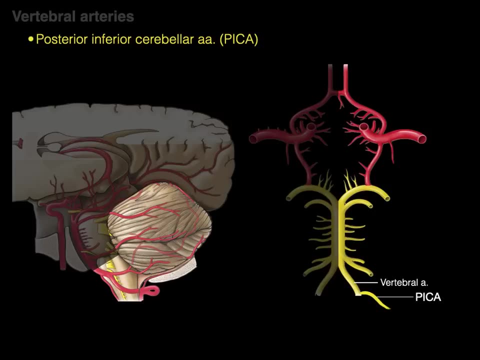 basilar artery. A branch of the vertebral artery is the pica, the posterior inferior cerebellar artery, which I've just drawn on there. So let's take a look at this lateral view and there is our cerebellum and there's the 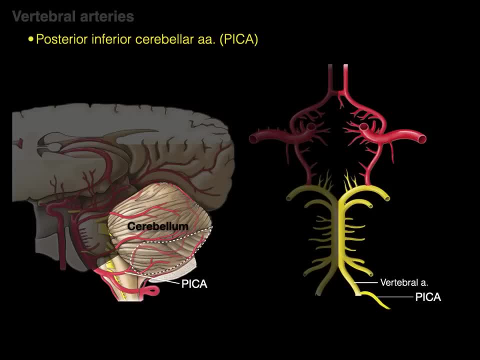 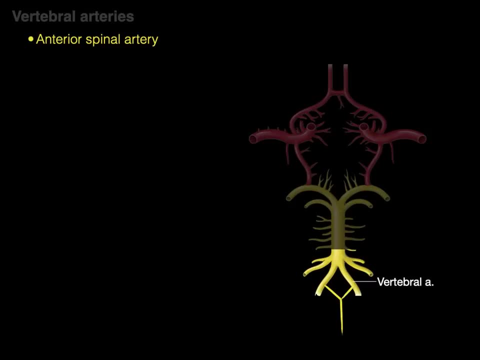 posterior inferior cerebellar artery, and there's the territory supplied, The bottom back of the cerebellum. We also have the anterior spinal artery. When we take our two vertebral arteries and we add the anterior spinal artery there, it then courses in front of the spinal cord. 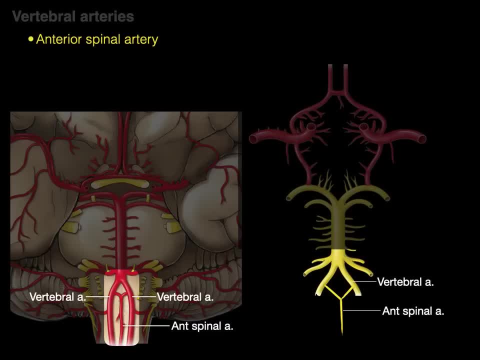 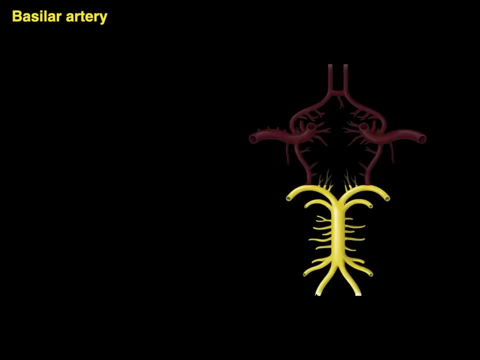 There's our two vertebral arteries and there's our anterior spinal artery. It supplies the front of the spinal cord. Now let's go to the basilar artery and its branches, And so the basilar artery is basically taking our two vertebral arteries and they come. 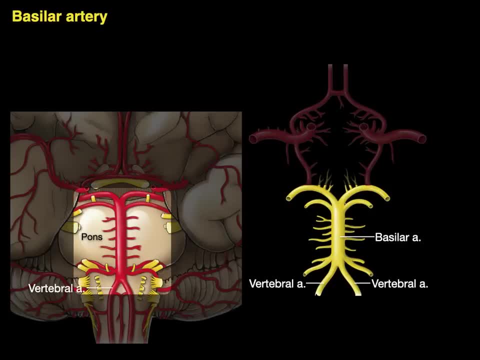 together to make the basilar artery. So here again. Here again is our two vertebral arteries and they come together to make the basilar artery that courses all along vertically along the pons, between the pons and the clivus. 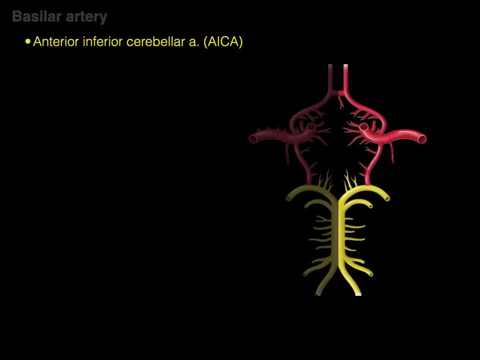 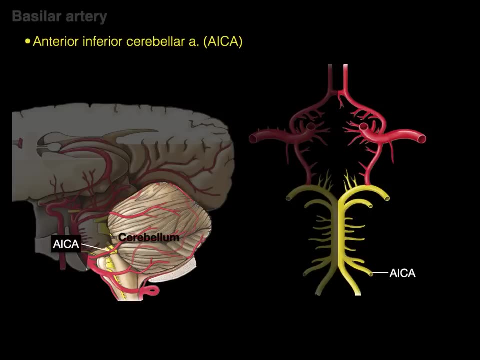 of the skull. Branches that come off include the anterior inferior cerebellar artery, there or the iaca, and there we have the cerebellum and there's the anterior inferior cerebellar artery. This supplies the front and bottom of the cerebellum. 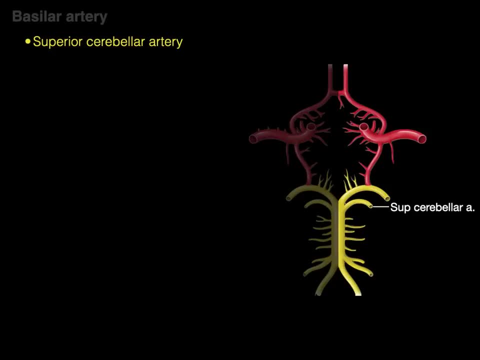 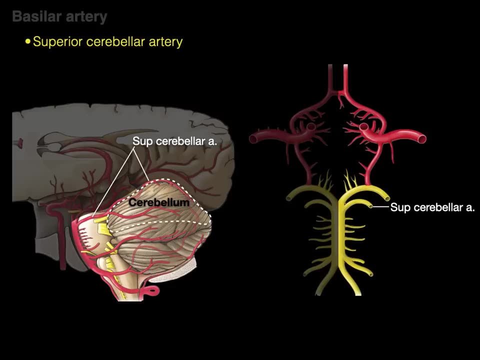 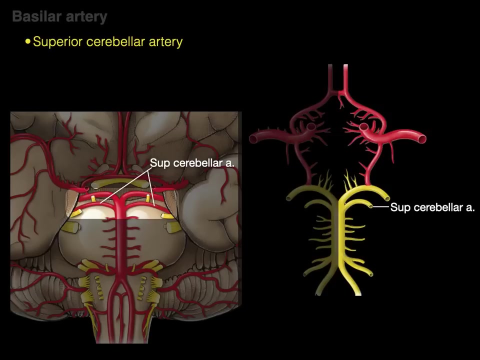 We also have the superior cerebellar artery that's more rostrally located And there is our cerebellum and there's our superior cerebellar artery that supplies the top of the cerebellum And there we have the superior cerebellar arteries, also shown in this view. 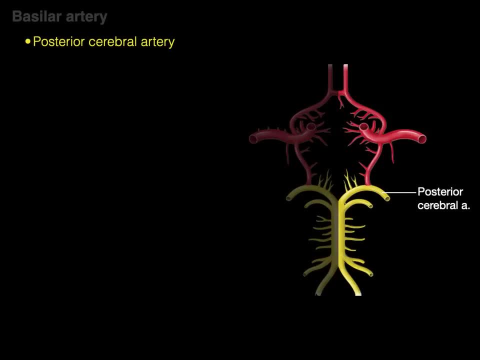 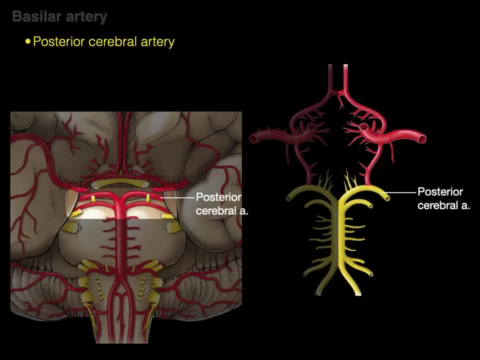 Then the very end of the basilar artery is showing the posterior cerebral artery, And the posterior cerebral artery is right there and it supplies the back of the cerebrum. Now I just want to take a little tangent for a second. 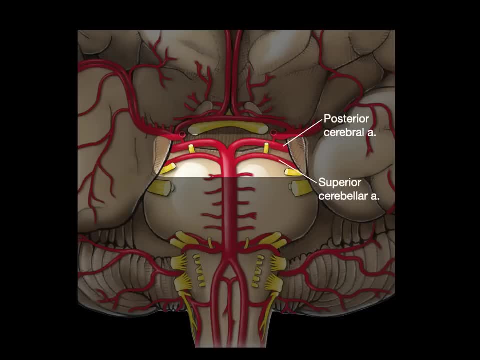 You see, there's the posterior cerebral artery And there's the superior cerebellar artery, Cranial nerve, three exits between the two of them. So if there's ever a baryaneurysm on the posterior cerebral or superior cerebellar artery, 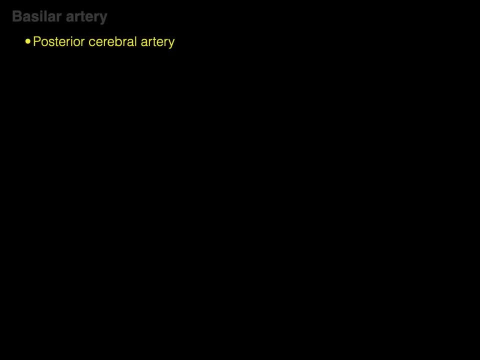 you can push on that cranial nerve three and have eye deficits, All right. So the posterior cerebellar artery's distribution is through the occipital lobe, our primary visual cortex, and to the temporal lobe, the posterior median portion and the inferior portion. 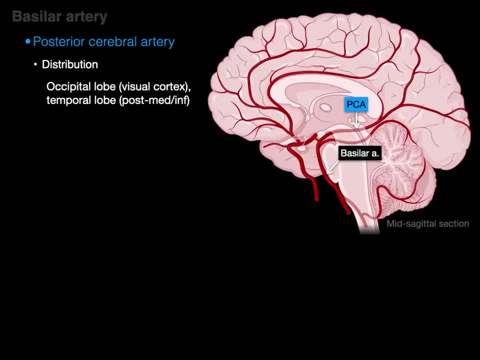 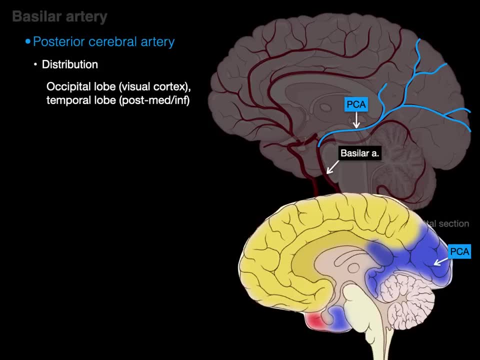 So here's a mid-sagittal section of the brain. There's our basilar and posterior cerebral artery And there is the distribution of the posterior cerebral artery. In this picture, the mid-sagittal view, the posterior cerebral artery in blue supplies the occipital lobe. 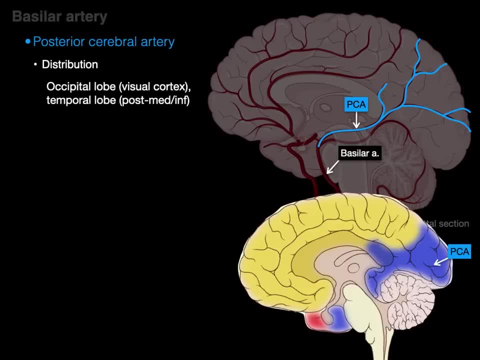 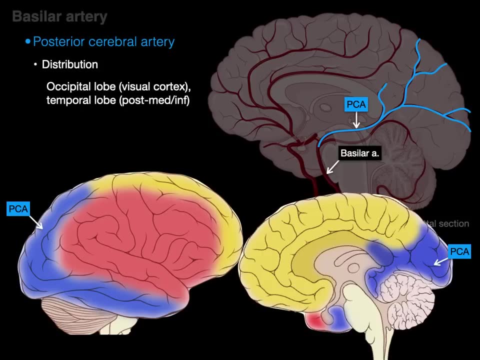 And then that posterior medial surface of the temporal lobe And in the lateral view you can see the posterior cerebral artery in blue supplying the occipital lobe and also the bottom or inferior portion of the temporal lobe. So now we've done the basilar artery. 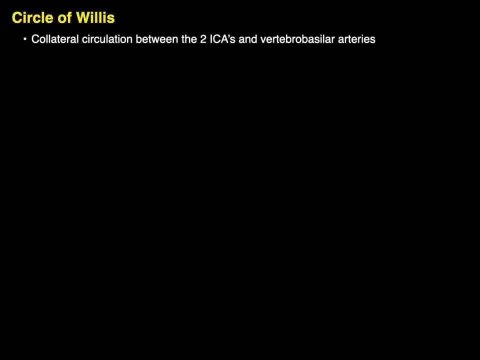 Let's talk about the circle of Willis. So what's the circle of Willis? Well, it's collateral circulation Between our two internal carotid arteries and the vertebral basilar arteries. So here we have that same picture: our two internal carotids and the basilar arteries. 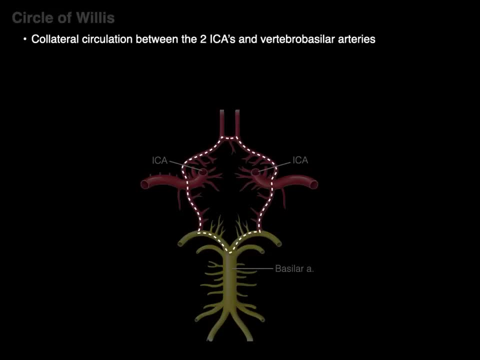 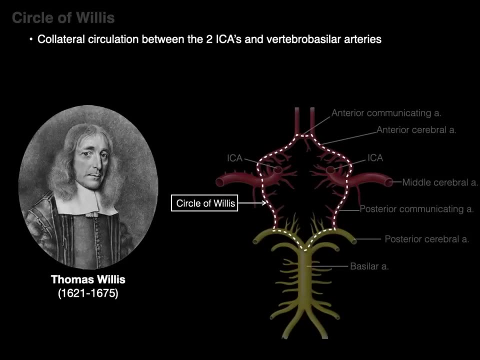 And then it's the collateral connection formed between those and our communicating arteries. That's the circle of Willis And it's named after this anatomist named Thomas Willis. He's from the 1600s. He named the circle of Willis. 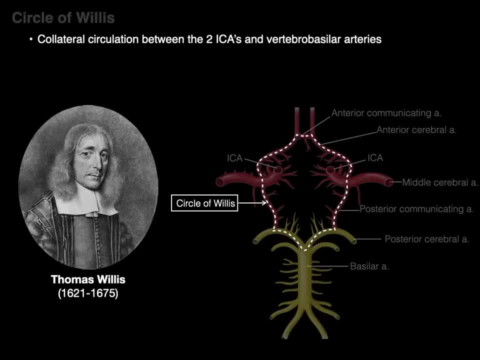 He also is one who numbered our cranial nerves 1 through 12.. We still do it. He actually also is the one who put the word mellitus and diabetes mellitus because he said, hey, that smells like honey, Let's call it the diabetes: a lot of urination that smells like honey. 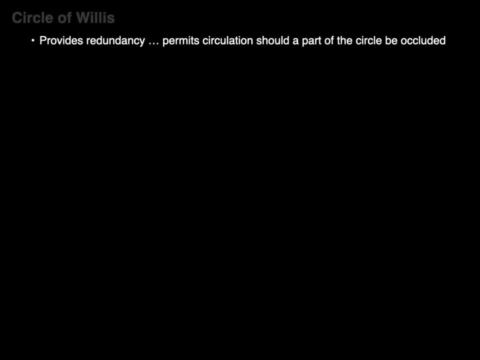 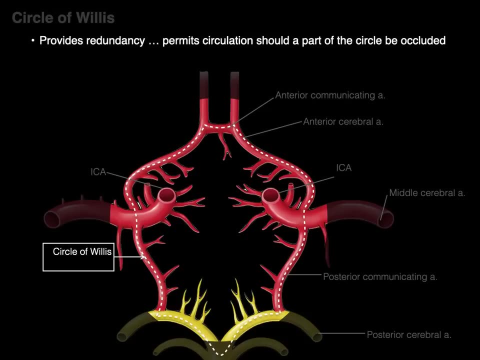 Okay, The circle of Willis provides redundancy. It permits circulation should a part of the circle be occluded. What do we mean by that? Well, here's that picture again. You can see the circle of Willis in that dast area. Now let's say that right, there is an occlusion of the anterior cerebral artery within the circle of Willis. 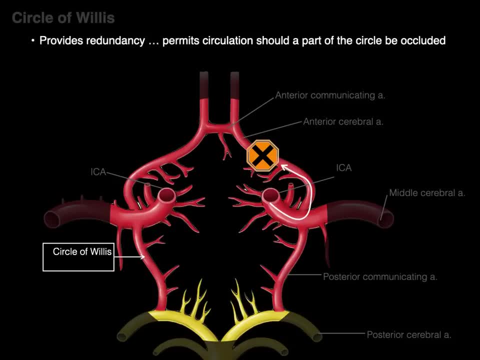 So blood comes up through the internal carotid artery and shing blocked, So blood on this side cannot get through to the anterior cerebral artery because it's blocked. But now watch that blood comes in from the contralateral internal carotid artery. 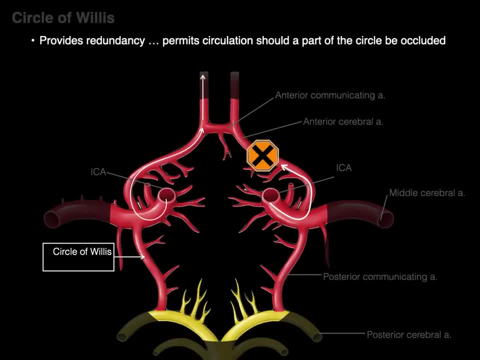 And then that blood can not only go to the anterior cerebral artery on its side, but also go across the anterior communicating artery and go up to the other side of the cerebrum, And so this circle of Willis provides redundancy within the circle. 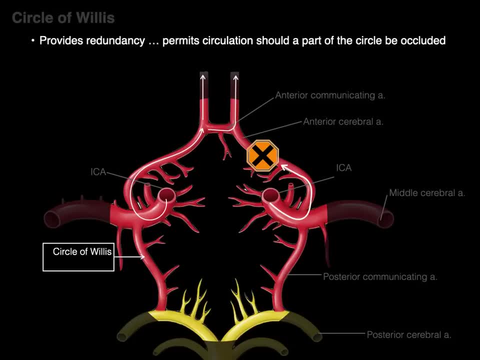 Now, if you go outside the circle, these terminal branches become empty. These are the end arteries. So if you block them, that's how you get ischemic stroke. But if you block within the circle of Willis, you can get this redundancy. 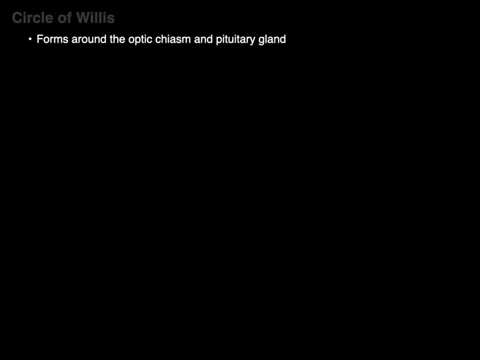 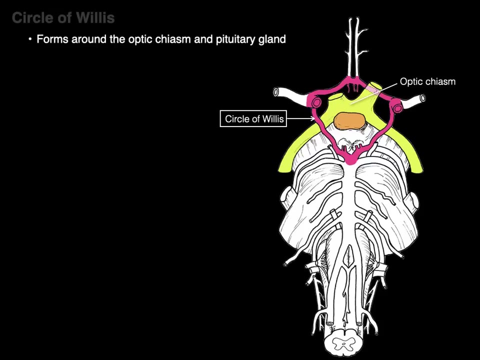 Pretty cool, right? And the circle of Willis is formed around the optic chiasm and pituitary gland. So there is a circle of Willis in red And then in yellow is the optic chiasm, which is the cross formed by our two optic nerves.